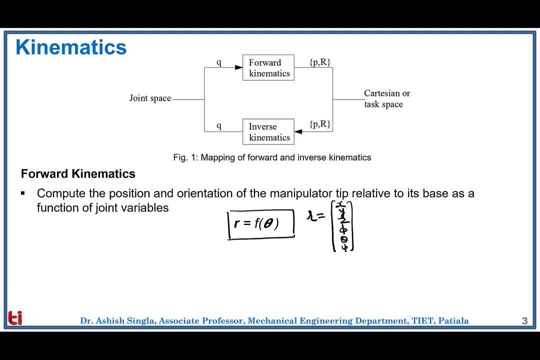 phi, theta, psi, the three orientation angles of the end effect, And theta represents a vector in joint space which contains all the joint variables. Let's say, for three degree of freedom, theta becomes theta1, theta2, theta3.. Next is the inverse kinematics in which given 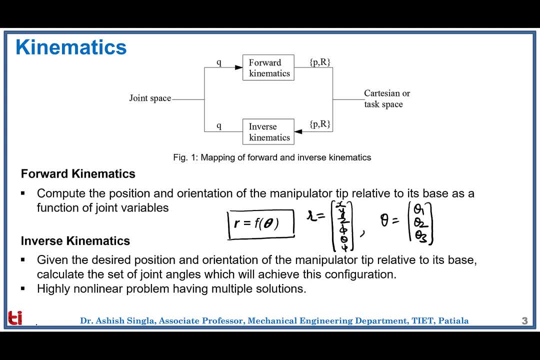 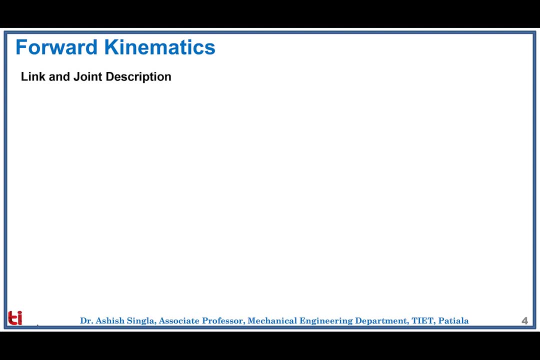 the desired position and orientation of the manipulator tip relative to its base, we need to calculate the set of joint angles which will achieve this desired configuration. Inverse kinematics is a highly non-linear problem having multiple solutions. So, first of all, about the link and 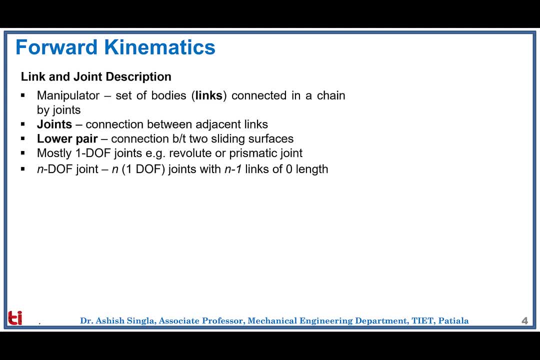 joint description. So any given manipulator can be represented as a set of bodies or links which are connected in a serial chains by joints, Where joints represents the intersection between two adjacent things, like shown in this figure. Six different kinds of joints are shown, So the first one shows the revolute joint, which is a single degree. 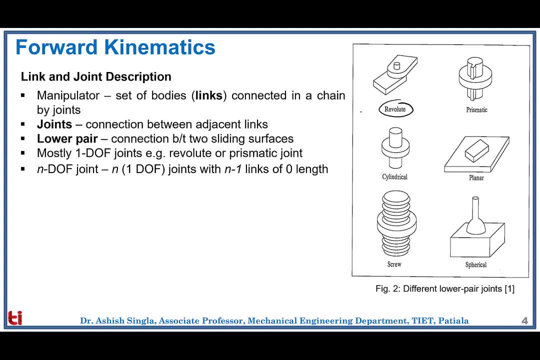 of freedom joint representing the rotation between two surfaces. The next one is the prismatic joint, which shows the translation between two sliding surfaces. The next one is the cylindrical joint, which shows both rotation as well as translation along the same axis. So this represents the planar joint which. 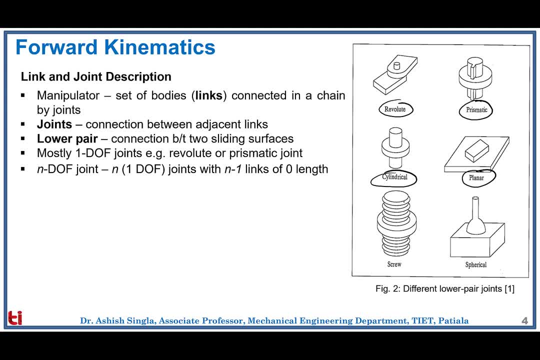 can represent the x-y movement as well as the orientation on the plane. The next one is the screw joint, which represents the translation as well as rotation along the same axis. So it's a two degree of freedom joint. And finally we are having a spherical joint which is like: 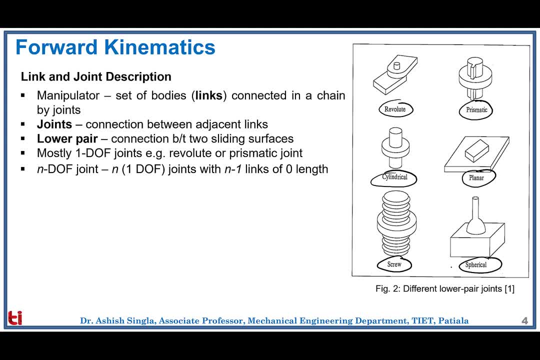 a ball and soccer joint having three degrees of freedom. So all these joints represent lower pairs where the surfaces are sliding over each other And in robotics mostly one degree of freedom. joints are considered either revolute or radial For prismatic joints, and if any joint have more than one degree of freedom, it can be. 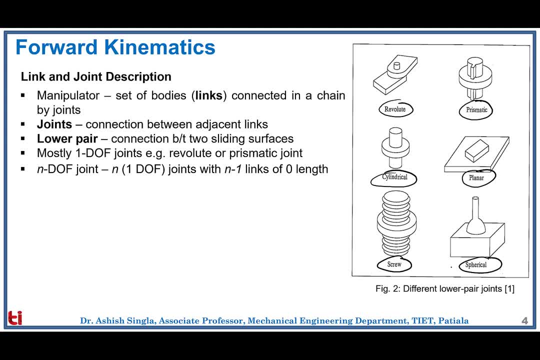 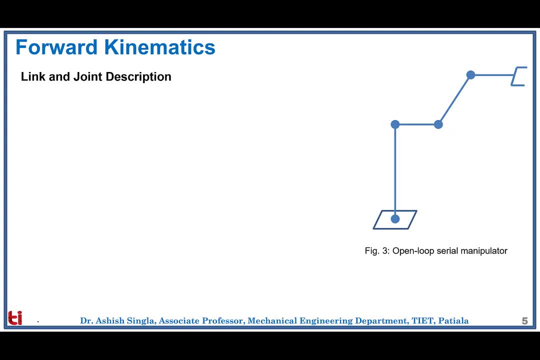 represented with the help of n joints with n-1 links of zero length. The figure shows the schematic diagram of a open loop serial manipulator which represents a open chain type structure, And in this this part is called as the base, or it is called 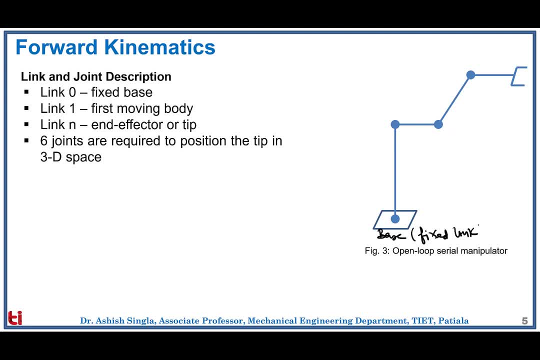 as the fixed link And it is being represented like L0.. And the next moving link is called as L1.. Then next is L2, L3, L4. And the first joint is written as J1, joint 2, joint 3, joint 4.. And the last portion, this is called as: 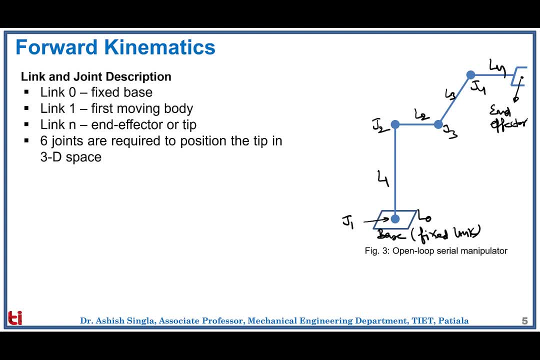 the end effector. Now, here you can see if we take this kind of a pair. So we are having a joint 2 followed by link 2.. Joint 3, followed by link 3, and joint 4 followed by link 4.. 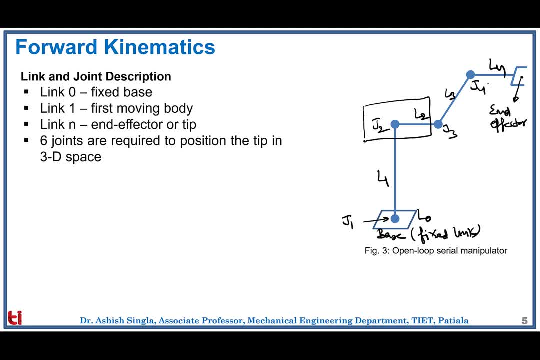 So link 0, as mentioned, is the fixed link and link 1 is the first moving link And link n is the n-th link, which represents the end effector or the tooltip, And in order to position the manipulator tip in this 3D space, 6 joints are required. 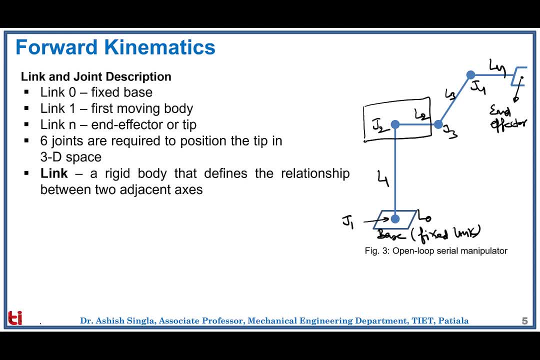 Next comes the description of link, which represents a rigid body that defines the relationship between two adjacent joints. So the description of link 1 represents a rigid body and the adjacent axis. so here you can see any. you can consider any link, like link l3, which defines the 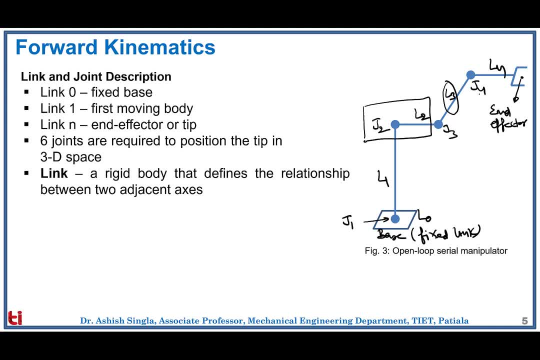 interconnection between j3 and j4. joint axes are lines in space. for example, the ith joint axis is the line about which ith link rotate, about i minus 1th link. now, just as there is a joint connecting two links, there is a link connecting two joints. in order to understand the forward, 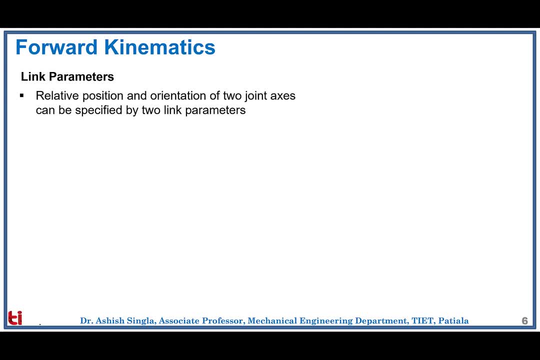 kinematics, we need to understand two kind of parameters: link parameters and joint parameters. first of all about link parameters, which represents the relative position and orientation of two joint axis. so here, let's say, we are having a link K which is interconnected with the help of two. 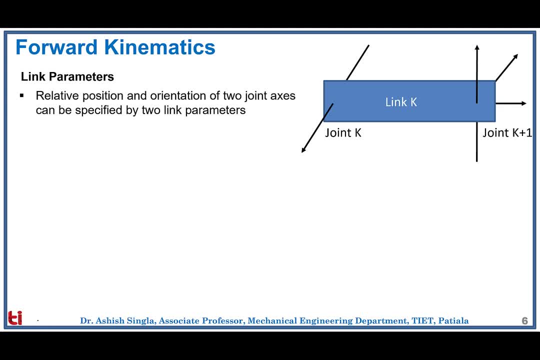 joints: joint K and joint K plus 1. so let's say this is ZK axis representing the joint K and this is the ZK K plus 1 axis representing the K plus 1th joint. this is the X K plus 1. this is the Y K plus 1. 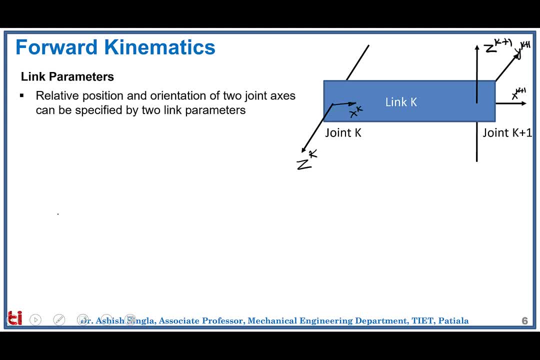 and let's say this is X- K. now, here you can see, the Kth link is interconnected with the help of two joints: joint K and joint K plus 1. so in order to establish the relationship between these two joint axis, two parameters are required. the first parameter is called as the link length, which is 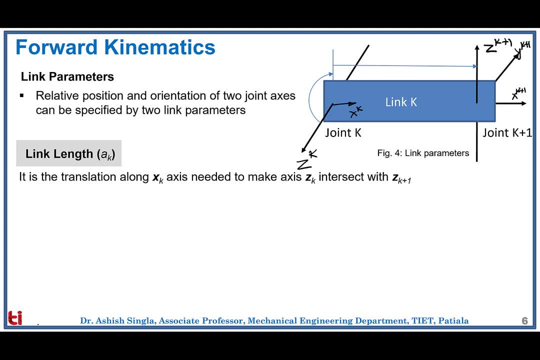 represented with the help of four: a K, which represents the translation along X, K axis which is needed to make X is Z K intersect with Z K plus 1. so here is X is Z K, this is the X is Z K plus 1. so if we move this coordinate from along this direction by this amount, a K, so the Z Kth joint. 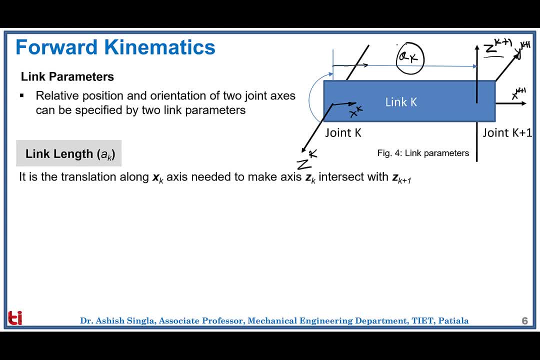 axis will intersect with Z K plus 1, so this is called as the Kth link length. the next link is the link twist angle, which is represented by alpha K. that represents the rotation between the two joint axis. formally it is the rotation about X K axis which is needed to make Z K axis parallel. 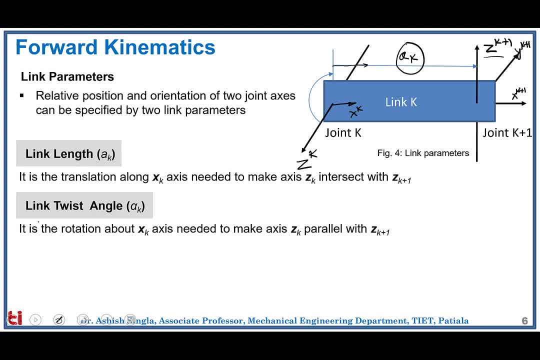 with Z, K plus 1, so we are talking about this angle, alpha K. then, regarding the first and last link, as per the conventions described, it can be clearly seen that the first and last link, length and twist angle, both are zero. both the link parameters are always constant and can be. 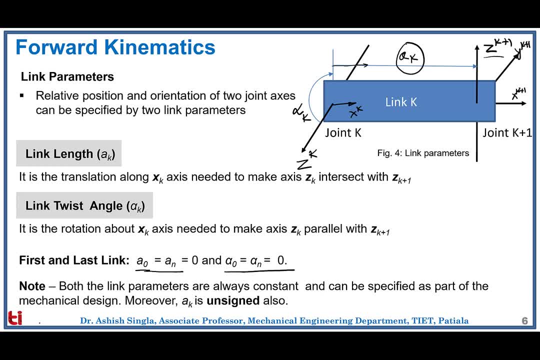 specified as a part of the mechanical design of the manipulator because, as the design is ready, the link length and twist angle are not going to change. and finally, the link length is unsigned also because link length represents a physical quantity which cannot take a negative value, whereas the link twist angle can take positive as well as negative. 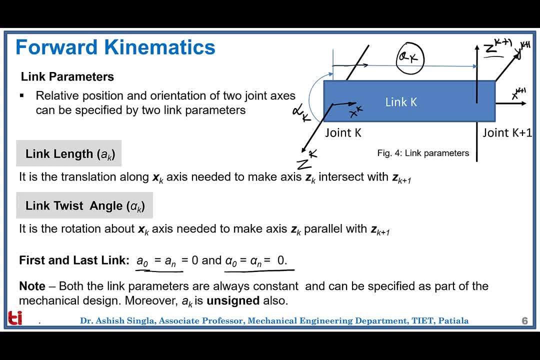 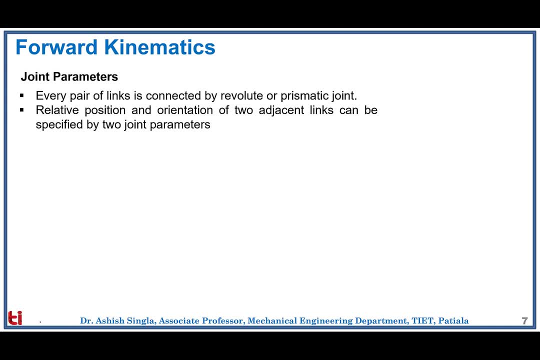 value depending upon the clockwise or counterclockwise rotation of the joint axis. next comes the joint parameters, where every pair of link is connected by either a revolute or a prismatic joint and the relative position and orientation of the two adjacent links can be specified by two joint. 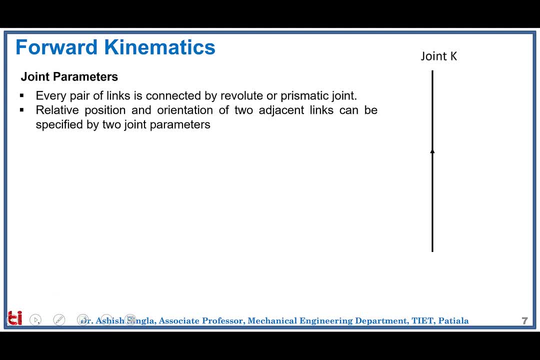 parameters, so which we can see here. so let's consider, we are having a joint K which can be represented with the help of a joint axis, Z, K, and this joint K represents the connection between link K and link K-1. so let's say this represents the XK axis and it represents 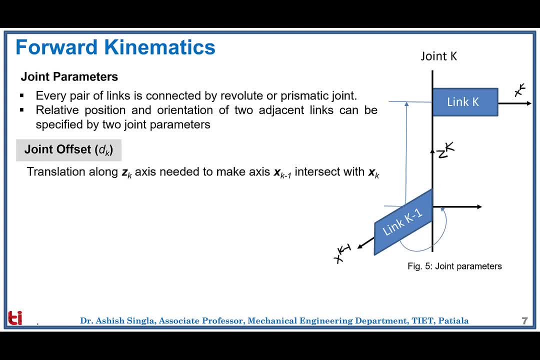 the XK-1 axis. so the first joint parameter is known as joint offset, TK, which represents the translation along ZK axis, which is needed to make XK-1 axis to intersect with XK axis. so this is the translation which is represented as DK, and the next is the joint angle, theta K, which represents the rotation. 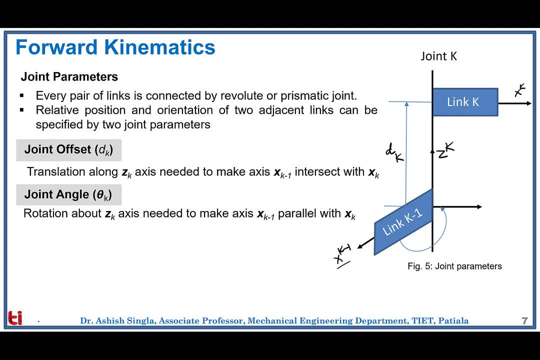 about ZK axis needed to make X is XK-1, parallel with XK, so this is the angle theta. so DK and theta K represents the two joint parameters which can take any values, positive or negative, again based on the convention used the first and last link for prismatic joint D1 and D and 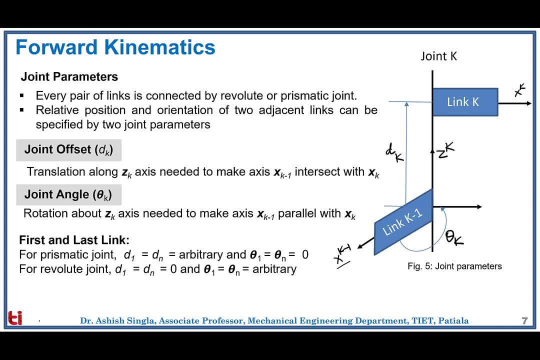 will be arbitrary and theta 1 and theta n are zero. and for revolute joint, D1 and Dn are zero, theta 1 and theta n are arbitrary. and finally, depending upon whether the particular joint is revolute or prismatic, one of the joint parameter will remain fixed and the other is variable. for example, if we 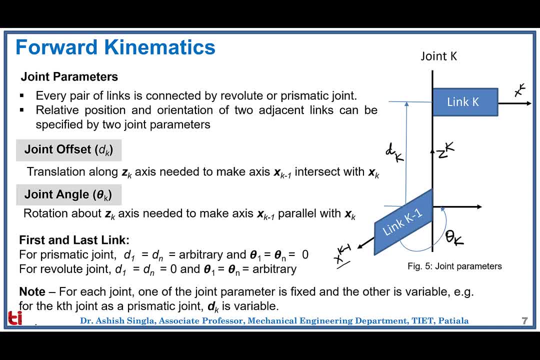 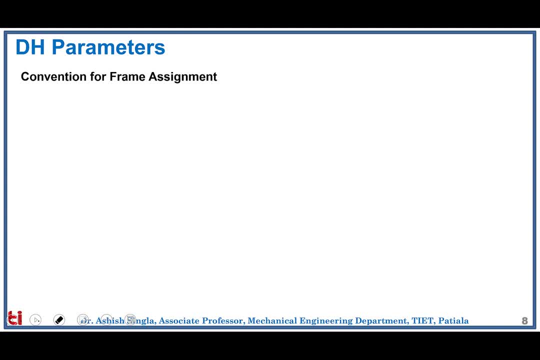 have a kth joint axis which is taken as a prismatic joint. DK is variable, whereas theta K remains fixed. in order to establish the kinematics, we need to rigidly assign the frames on each moving part. so first of all we need to discuss the frame assignment conventions. so let's consider a three degree of freedom manipulator. so 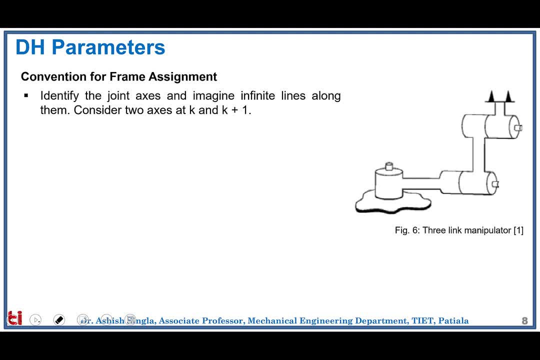 the first step is we need to identify the joint axis and imagine infinite lines among them. so let's say the first line, a second line and third line, and let's consider two such axes as axis K and K plus one. next is we need to identify the common perpendicular or point of. 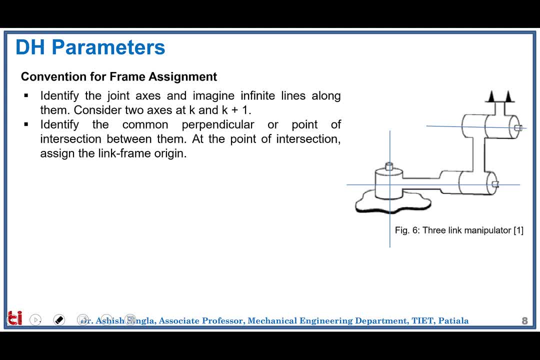 intersection between them. and at the point of intersection we assign the link frame origin. so here you can see, is the first two lines, this is the point of intersection. so we can say this is one of the origin, and second and third axes are parallel, so there is a common perpendicular. 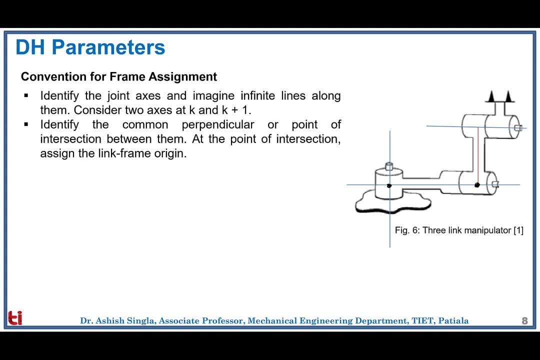 this red line and over here we can mark the origin of the second frame, assign the zk-axis pointing along the kth joint axis. so this we can say this is zk- or the joint matrix, matrix of zk- and we can, and let's say upwards, and this is z, k plus 1. next is a sign: x, k, x is pointing along the common. 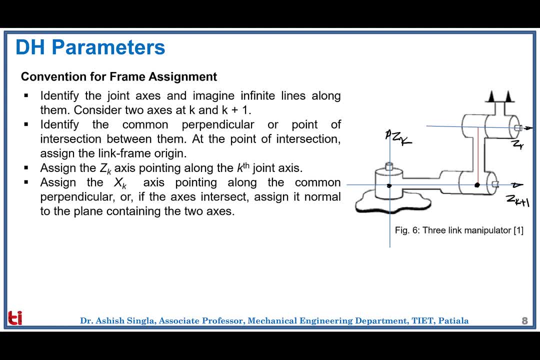 perpendicular. so let's say this is z? k plus 2, so as z k plus 1 and k plus 2 are parallel, so there is a common perpendicular. so this represents the direction of x, k plus 1. and in the case when the two joint axes are intersecting, like z? k and z k plus 1, which are intersecting over here, x, k. 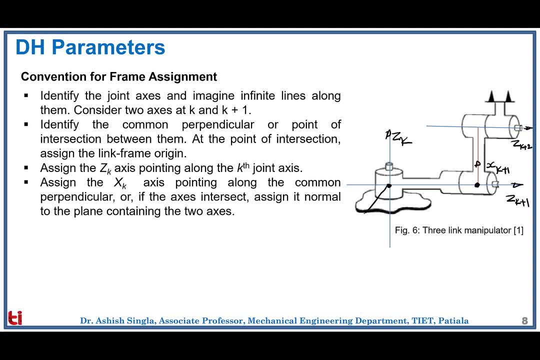 will be assigned in a direction perpendicular to the plane of both axes. so this is the direction of x k. and finally, we can assign y to complete the right hand coordinate system. so here you can see, for the kth frame, this is the direction of y k, because if you curl your fingers from x k to y k, 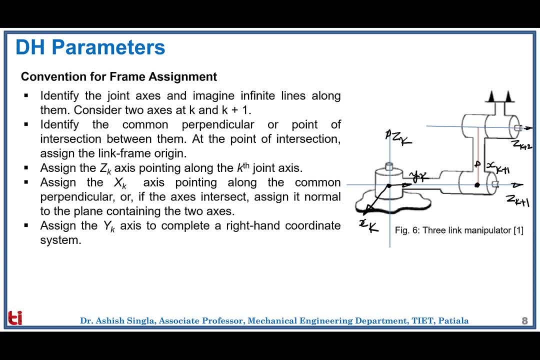 thumb points in the direction of z k. similarly for z k and z k plus 1. this is the direction of y k, because if you curl your fingers from x k to y k- k plus 1th frame, if we curl our fingers from z? k plus 1 to x? k plus 1, the thumb points in the 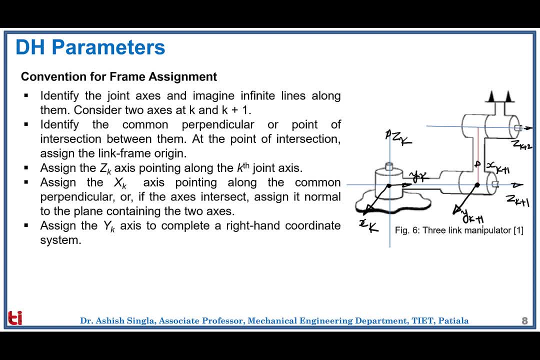 direction of y, k plus 1. so this is how we can complete the frame assignment and finally, we can assign a zero frame for the fixed base to match with frame 1 when the first joint variable is zero, and we can assign frame n at the end effector of the manipulator and we can choose. 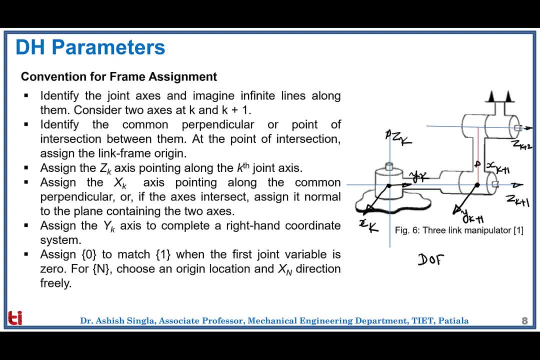 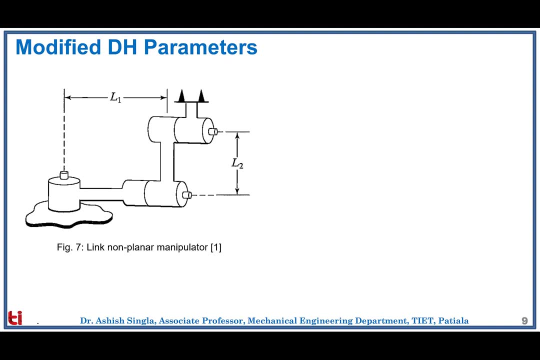 its xn direction freely. so for three degrees of freedom robot we need to have five frames. so in general we have n plus two frames for solving the forward kinematics of a n degree of freedom robot. so next we can see that the frame assignment is not unique. 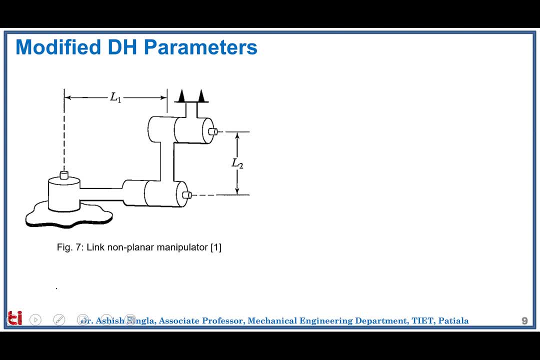 so we can have different frames and accordingly the link parameters and joint parameters are different. so this is the original frame assignment in this figure. so here you can see, we have the freedom to choose z axis. this z could be up or down the frame assignment, so we can choose z axis. 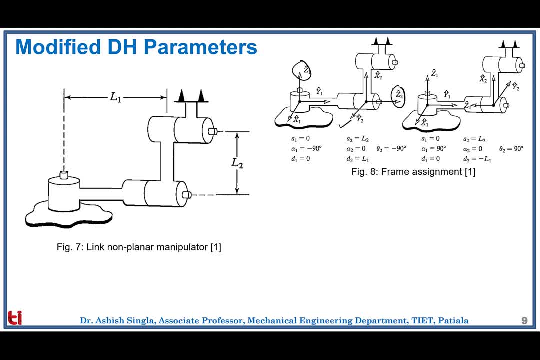 or this z could be towards the right or towards the left. so in the next figure we can see we can choose the second frame to be like this, where the z points towards the left. now, accordingly, all the link and joint parameters will change. we have two more options. so in this you can see: 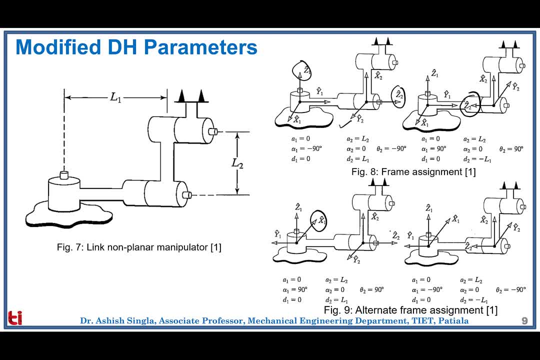 x1 is taken inside the plane of the board with z1 towards the right, and in the last figure we can see x1 is again taken in the plane of the board where z2 is taken towards the left hand side. so there are many options in which we can assign the frames which. 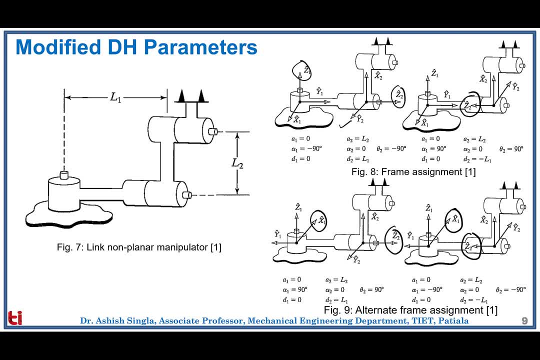 justifies that frame assignment is not unique. but in the end, whatever frame assignment we will do, if we have followed the conventions in a systematic manner, the end result, which is the description of the tool tip with respect to the base of the robot, that should come out to be seen. next comes the dh. 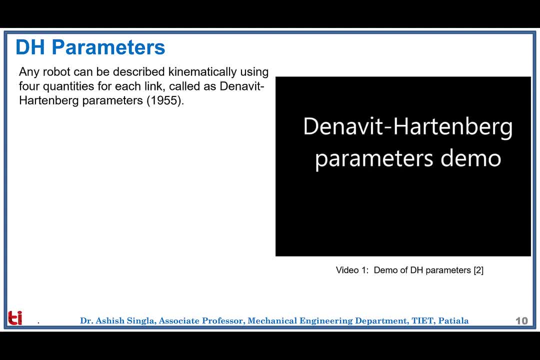 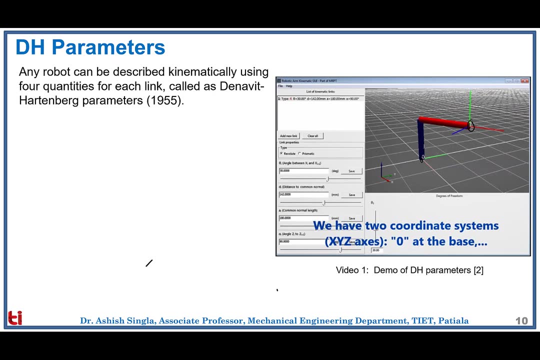 parameters which are developed by danowitz and hartenberg in 1955 and according to which four parameters are assigned for each link, which we can see in this video. consider this one degree freedom robot, where two frames are assigned: frame 0 and frame 1. frame 0 is assigned at the base of the 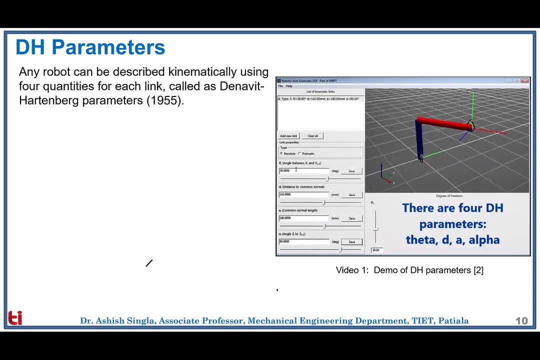 robot and frame 1 is assigned at the tip of the robot and there are four parameters which are used to establish the relationship between frame 1 and frame 0. all these four parameters can be changed with the help of these four bars. so the red one bar represents the common normal, the blue one represents the distance along the previous z. 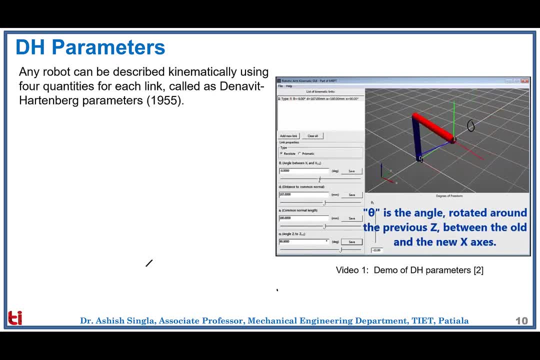 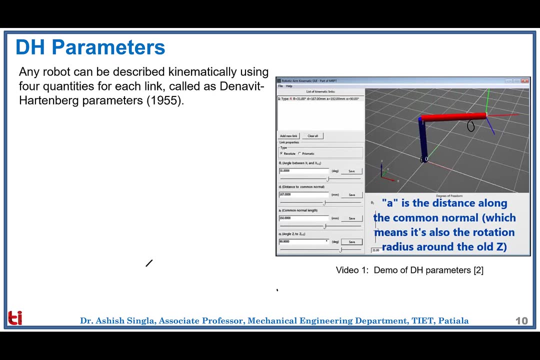 where theta is the angle rotated about the previous z. here we can see from the top view also. so this is the angle theta rotation about the previous z axis. so this is you can see the link length, the distance along the common normal. and finally, alpha represent the rotation between. 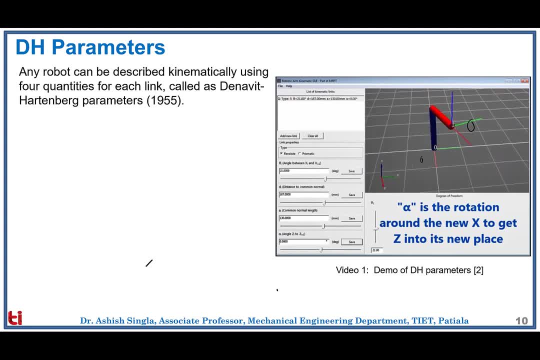 the two z axis. as you change the value of alpha, you can see the frame 1 rotates, which shows that the angle between the two respective z axis keeps on changing. so this is basically to understand what are these four parameters and how they are going to affect the relationship between the two frames. in order 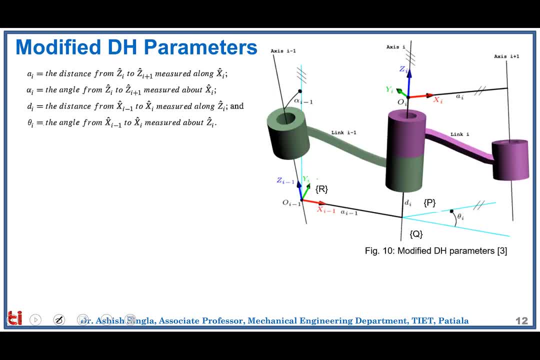 to map the ith frame to i minus oneth frame. let's define three intermediate frames, that is, frame r, frame q and frame p, and let's try to understand how they are different from the other frames. the frame r is different from i minus one frame, in the sense that both have 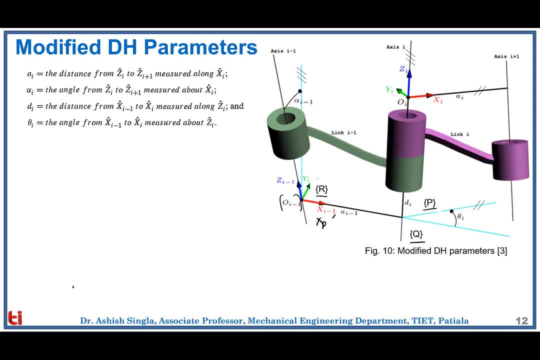 same x axes, that x, r and x i minus one are in the same direction but their z axes are different. so ZI-1 is along the I-1th joint axis where ZR is along the I-th joint axis. So the basic difference between these two frames is the angle alpha I-1.. 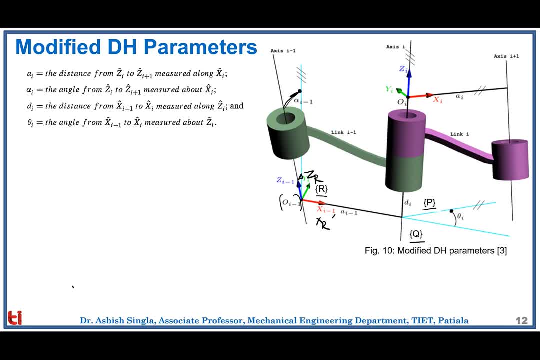 Next comes the Q-frame. The Q-frame and R-frame have same X and Z directions, But the Q-frame is translated from the R-frame by AI-1 in the direction of XX. Next comes the P-frame, where both P and Q have same Z axis. 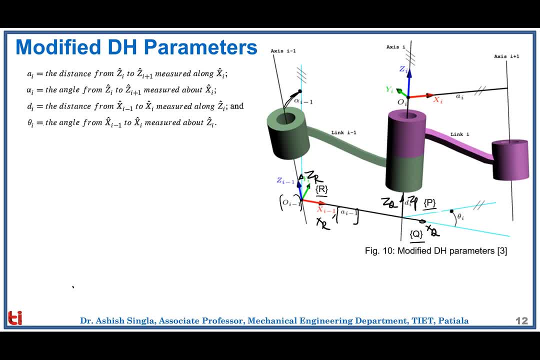 So ZP is also in the same direction. However, the XP and XQ are different by the angle thetaI, so which means that the p-th frame is rotated about Z-axis by angle thetaI. And, finally, the p-th frame and ith frame have same Z as well as the same X axis. 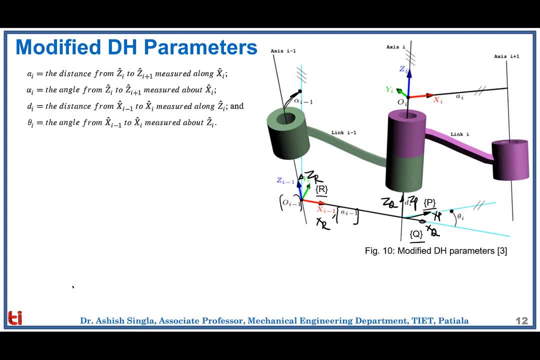 However, is translated from the pth frame by di amount in the direction of zi axis. So each frame will represent one of the dh parameters and we can write the mapping of ith frame to i-1th frame using these four frames like this way, where pi is a point defined. 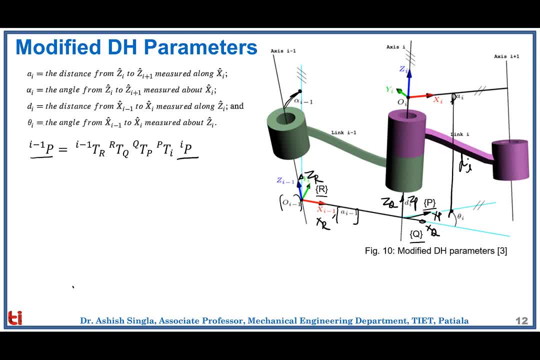 in ith frame and pi-1 is point defined in the i-1th frame. So the first transformation will map the ith frame to pth frame, then pth frame to qth frame, qth frame to rth frame and finally rth frame to i-1th frame. 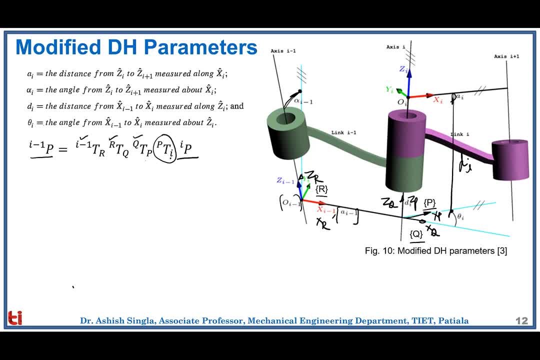 So, in nutshell, we can write this- all four transformation as a single transformation matrix. Further, we can write these transformation matrices in more simplified manner. So, first of all, let's about this transformation which represents translation along the i-th frame. So, first of all, let's about this transformation which represents translation along the zi axis. 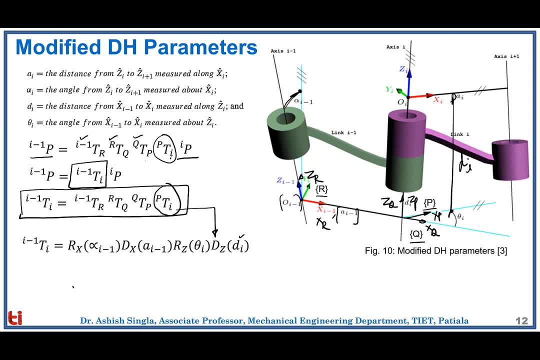 by amount di. Next comes the pth to qth transformation, which represents rotation about z-axis by amount theta i. Then qth to rth transformation, which represents the translation along the x-axis by amount ai-1.. And finally the rth to i-1th transformation, which represents the rotation about x-axis. 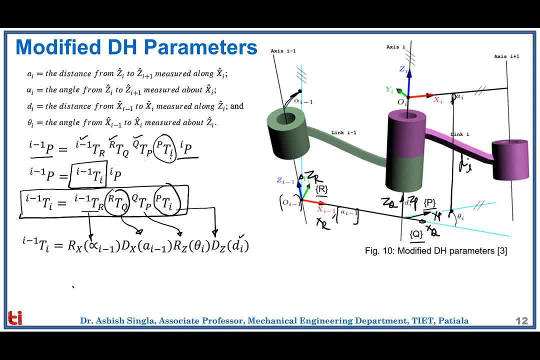 by amount. alpha i-1.. Here we can see that the first two transformations are about zi, The first two are about x-axis and the last two transformations are about zi. The first transformation represents the rotation, the next transformation represents the translation. So it's the rotation and translation along the same axis which can be written as a screw. 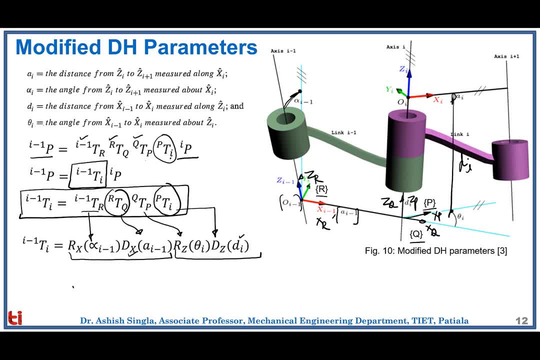 transformation, because in screw you can see that both translation as well as rotation of the screw happens along the same axis. So the screw transformations are commutative. either you can write the rotation first or the translation first. it's one and the same thing. 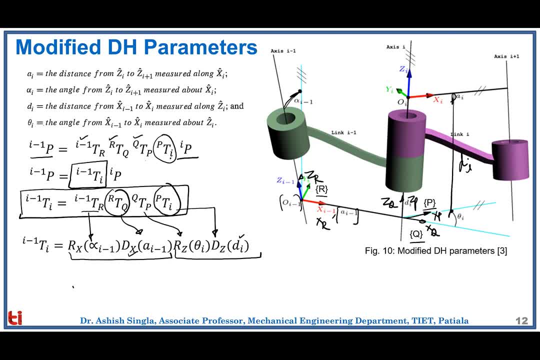 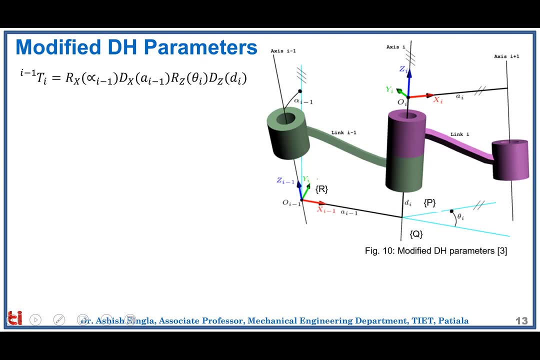 Similarly, we can write these two transformations about the z-axis as another screw. So finally, the mapping from i-th to i-1th frame can be written like these two screw transformations. Next, we can write these four transformations in expanded form. So let's say first about the dz di transformation, which represents only the translation along. 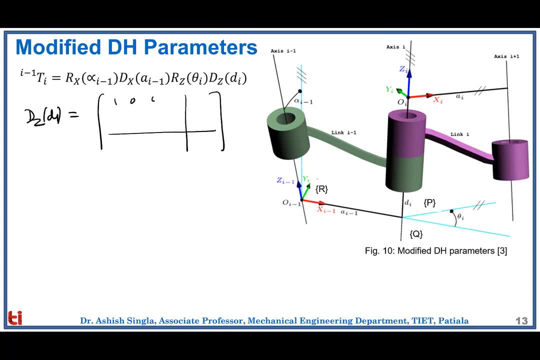 the z-axis. That means the rotation matrix is identity. last row is 0001 and it's the translation along the z-axis, so 00 di. Next comes the rotation about z-axis, which is written as rz, theta, i, So we can write this as a standard template of rotation about z-axis. 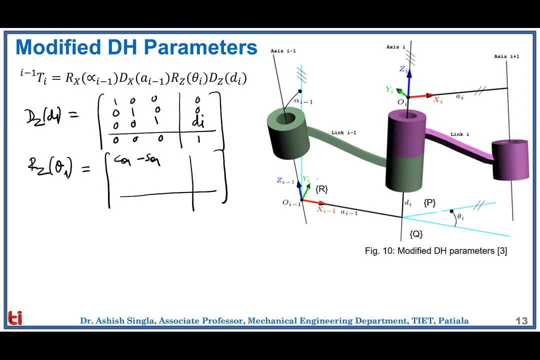 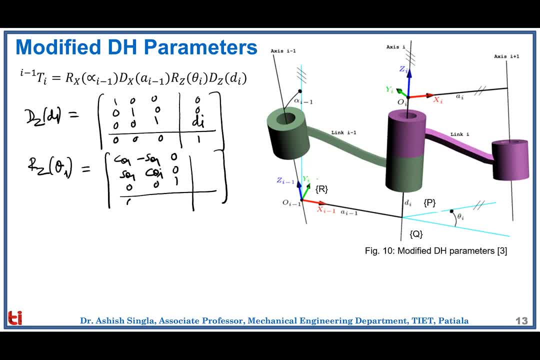 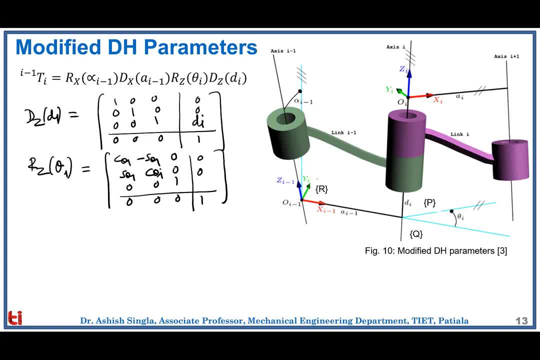 s theta i is 0.. s theta i is 0.. s theta i is c. theta i is 0.. mae theta i theta i: 0, 0001. last row is 0001 and the last column is 000.. Next comes the translation about x-axis by amount: ai-1.. 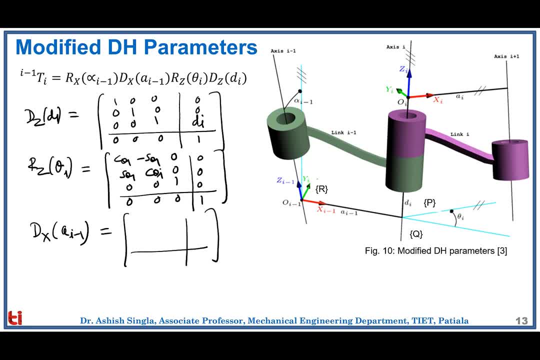 So again we can write the rotation as identity matrix: 1000, 1000 and the last row is 0001.. And the last column is ai-1.. b Kris- graduate math and Enterprise lectures six queuer card presentation 1: 6 about deep. 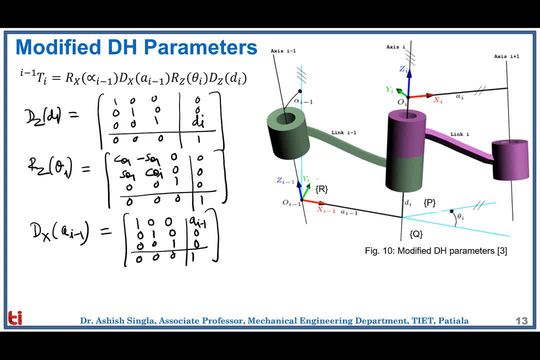 anomalies, protagonism, Plant trasnfaction, rausatnelight axis, autism with inactivated 0: 0 and finally we have the rotation about the x-axis amount is alpha e minus 1. so these are the four transformation matrices in expanded form. so when we 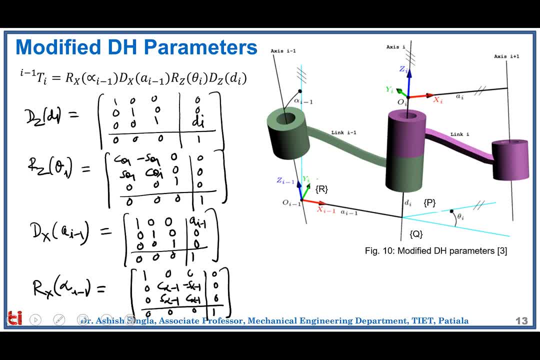 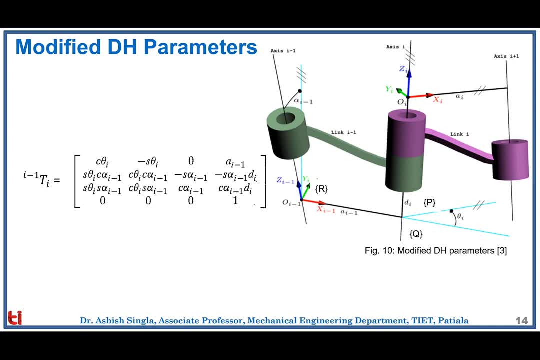 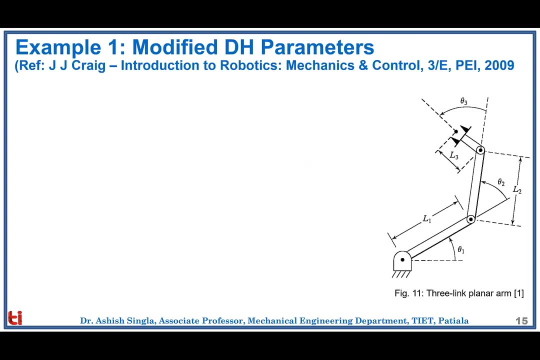 multiply them in order, we will get the final transformation matrix. like this way, and this matrix we have to apply iteratively to find out the final transformation from the tip of the manipulator to the base of the manipulator. next we will present one example which you can practice by starting with. 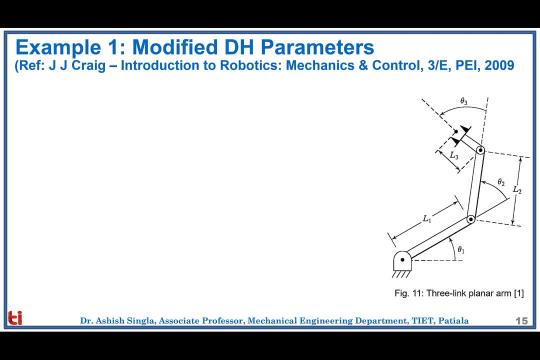 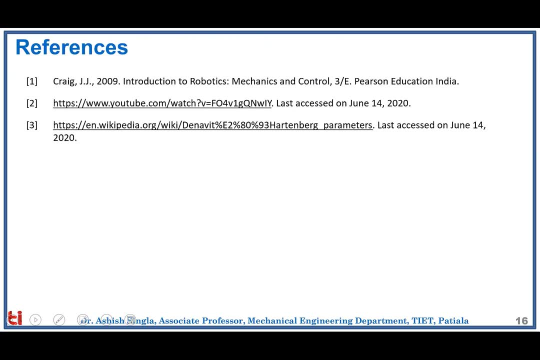 assigning the frames using the conventions and find out the DS parameter table, which should be like this way. so we will cover this example in detail in the next session. thank you, 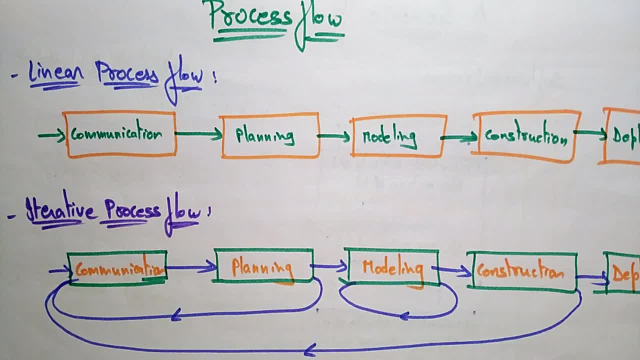 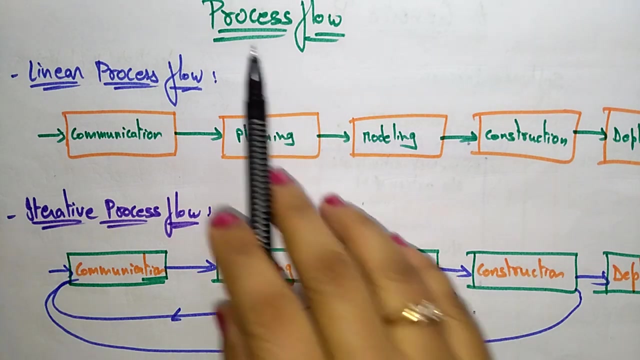 Hi students. coming to the next topic, that is, the process flow. Whatever the process you are taking, how that process is going to be flow. A process or you can take, or a product you can take, or a thing you can take, or whatever activity you are taking, you are dealing, So that has to be followed. some process means there is some flow. you have to process, you have to take place. That is a process flow. A process flow can be done in different ways.